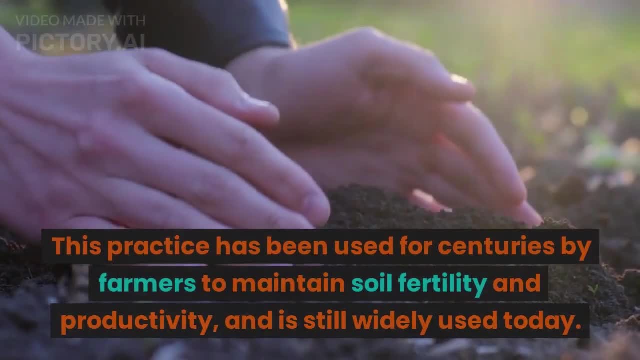 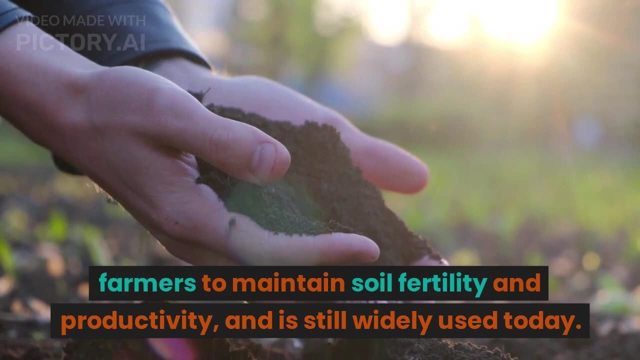 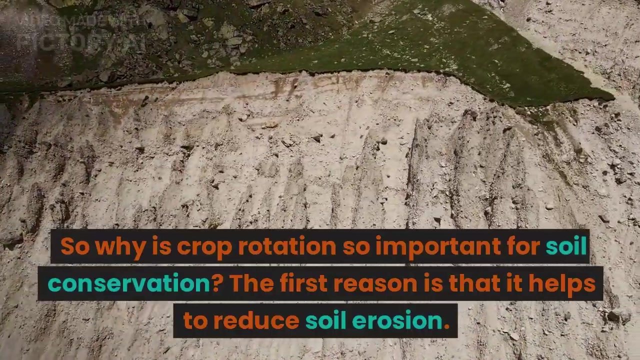 the same crop year after year. This practice has been used for centuries by farmers to maintain soil fertility and productivity, and is still widely used today. So why is crop rotation so important for soil conservation? The first reason is that it helps to reduce soil erosion. 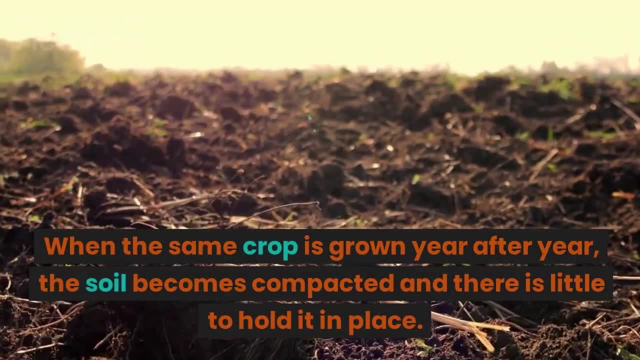 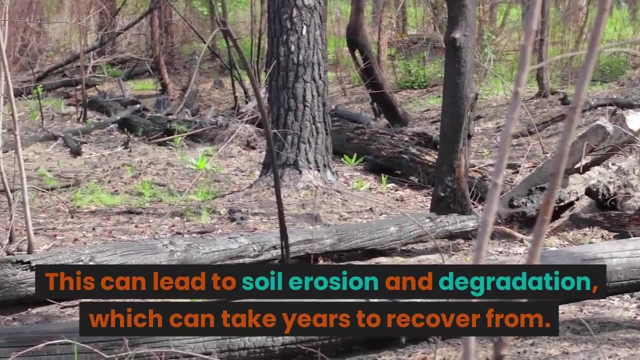 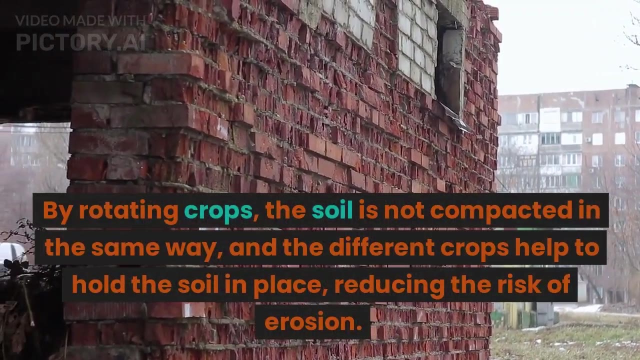 When the same crop is grown year after year, the soil becomes compacted and there is little to hold it in place. This can lead to soil erosion and degradation which can take years to recover from. By rotating crops, the soil is not compacted in the same way and the different crops help to. 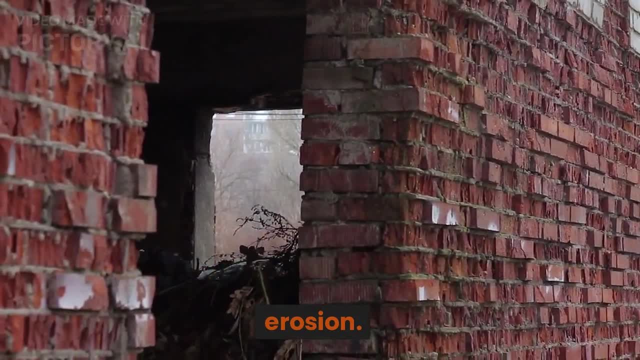 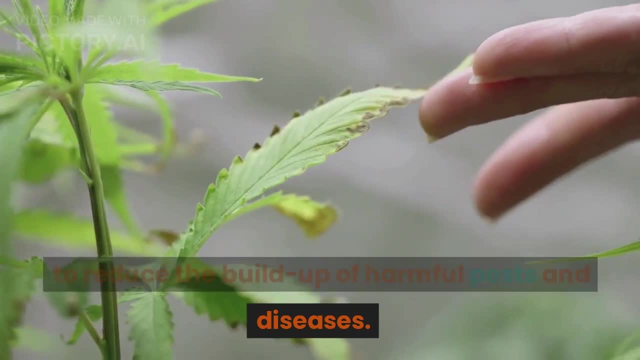 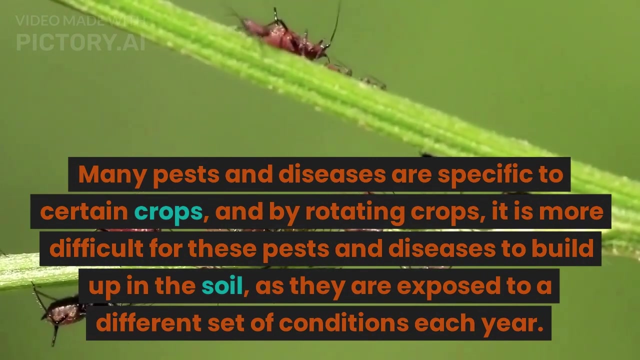 hold the soil in place, reducing the risk of erosion. Another benefit of crop rotation is that it helps to reduce the buildup of harmful pests and diseases. Many pests and diseases are specific to certain crops and by rotating crops it is more difficult for these pests and diseases. 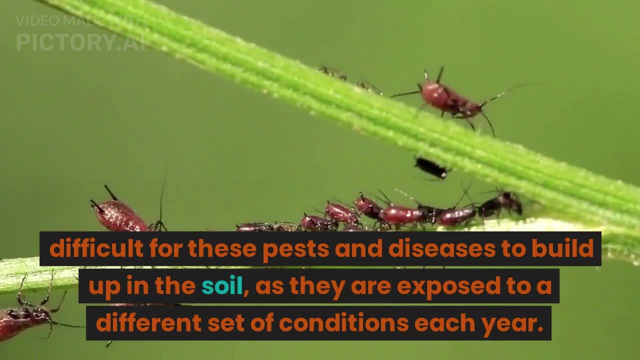 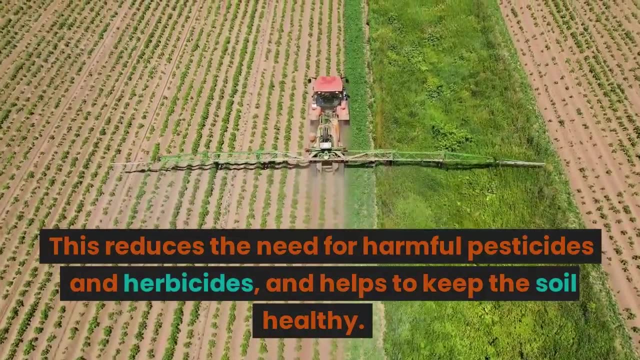 to build up in the soil. Crop rotation is the practice of growing a series of crops in the same soil, as they are exposed to a different set of conditions each year. This reduces the need for harmful pesticide and herbicides and helps to keep the soil healthy. Crop rotation also helps. 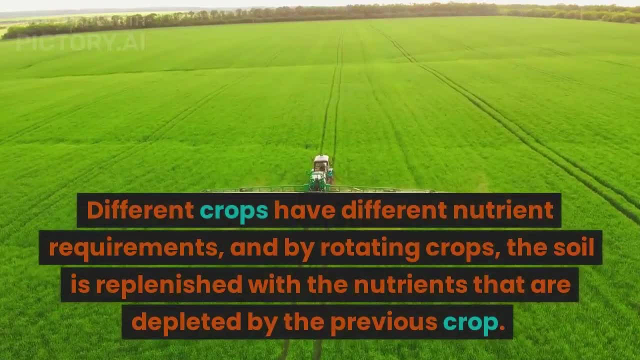 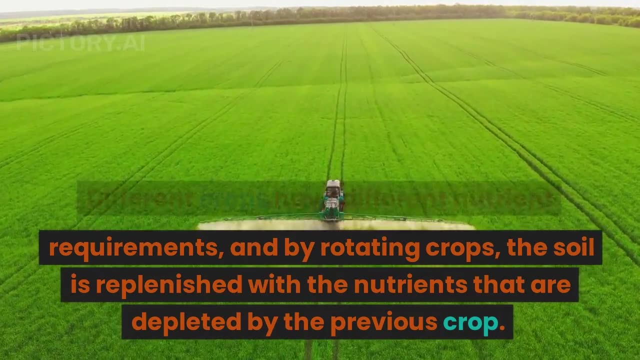 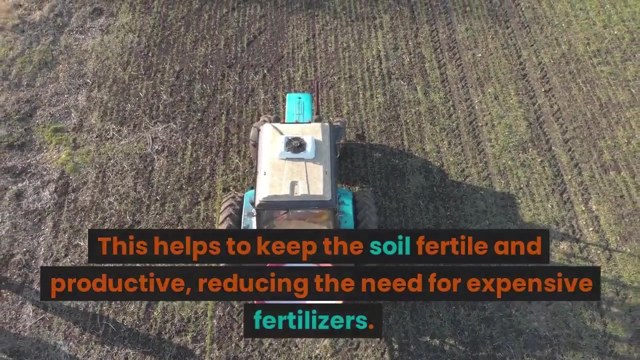 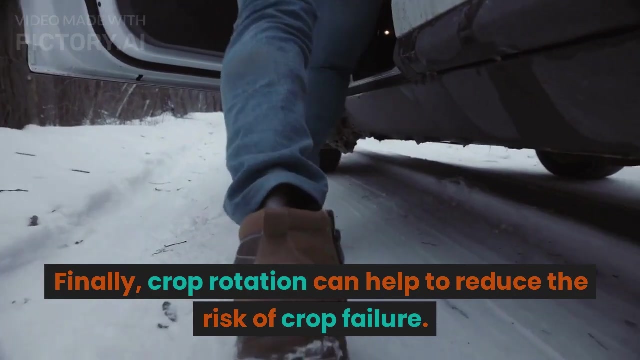 to maintain soil fertility. Different crops have different nutrient requirements and, by rotating crops, the soil is replenished with the nutrients that are depleted by the previous crop. This helps to keep the soil fertile and productive, reducing the need for expensive fertilizer. Finally, crop rotation can help to reduce the risk of crop failure When the same crop is grown year. 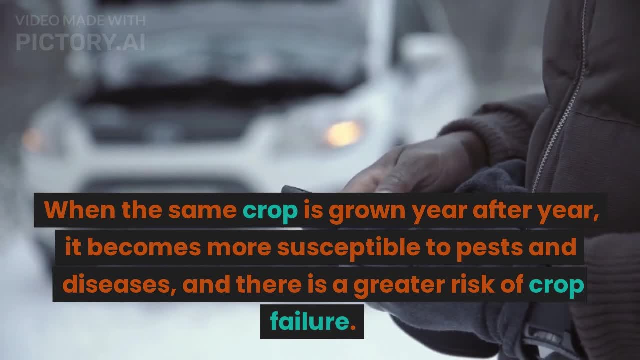 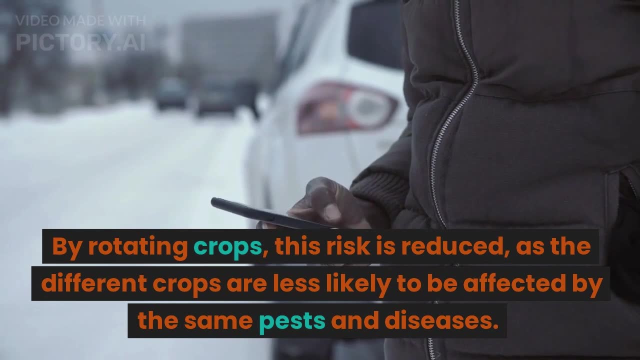 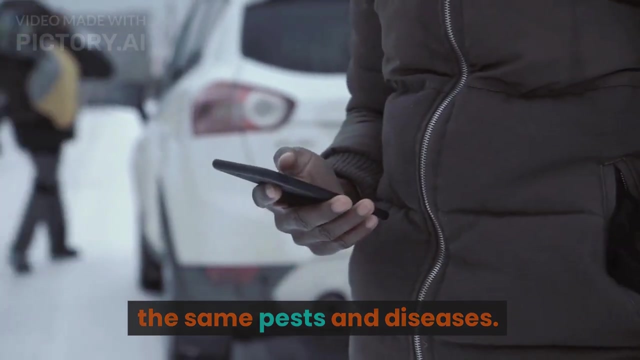 after year, it becomes more susceptible to pests and diseases and there is a greater risk of crop failure. By rotating crops, this risk is reduced, as the different crops are less likely to be affected by the same pests and diseases. In conclusion, crop rotation is a simple but effective